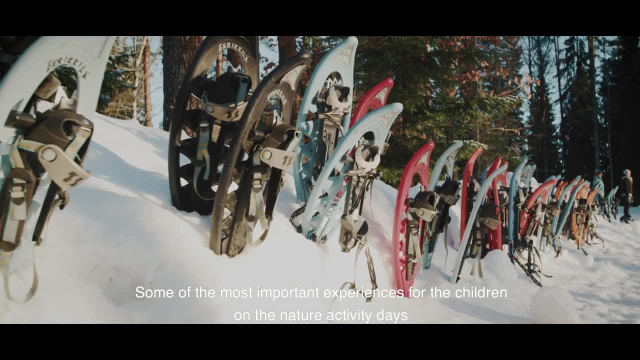 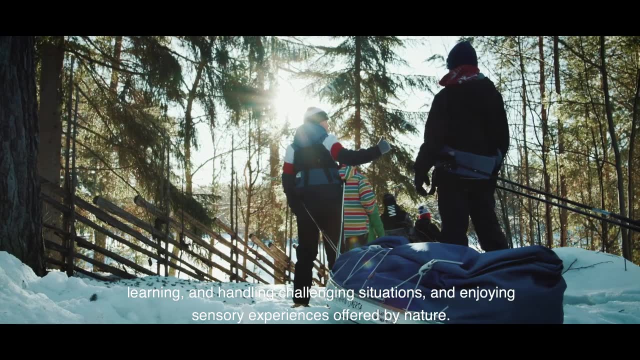 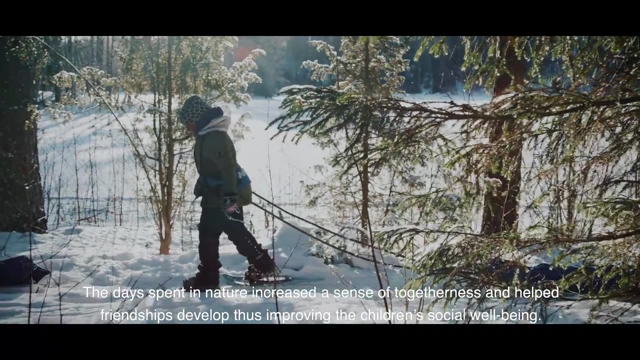 most important experiences for the children on the Nature Activity Days involved being together and cooperating with classmates, a sense of freedom, learning and handling challenging situations, and enjoying sensory experiences, often by nature. The days spent in nature increased a sense of togetherness and 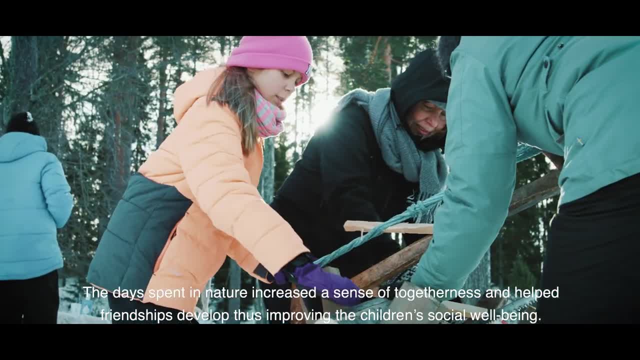 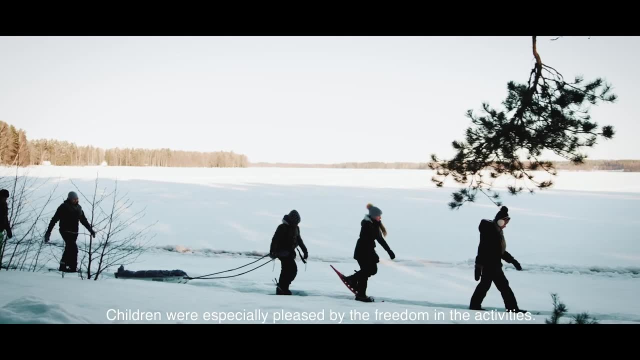 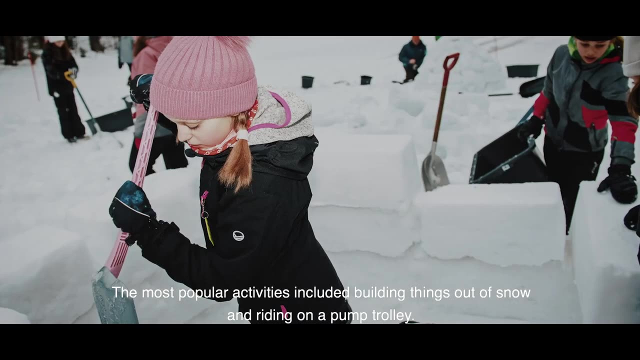 helped friendships develop, thus improving the children's social well-being. Children were especially pleased by the freedom in the activities. The most popular activities included building things out of snow and riding on a pump trolley. In them, the children experienced the freedom to do things and the joy of. 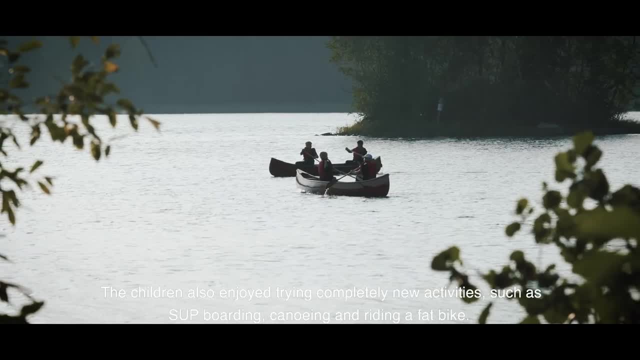 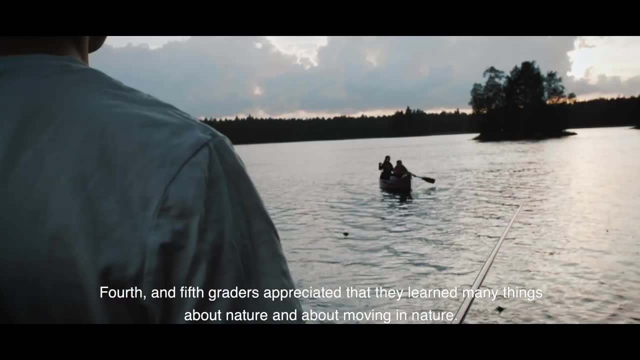 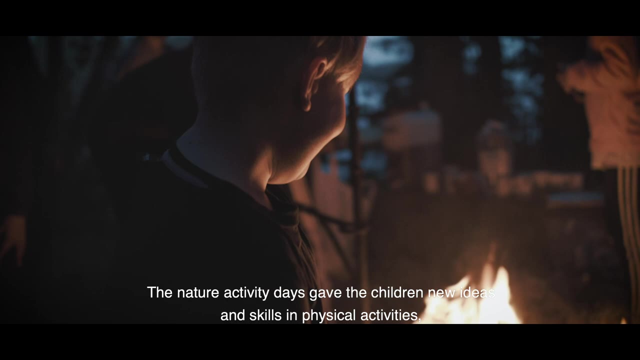 working together. The children also enjoyed trying completely new activities such as SUP boarding, canoeing and riding a fat bike. Fourth and fifth graders appreciated that they learned many things about nature and about moving in nature. The nature activity days gave the children new ideas and skills in physical 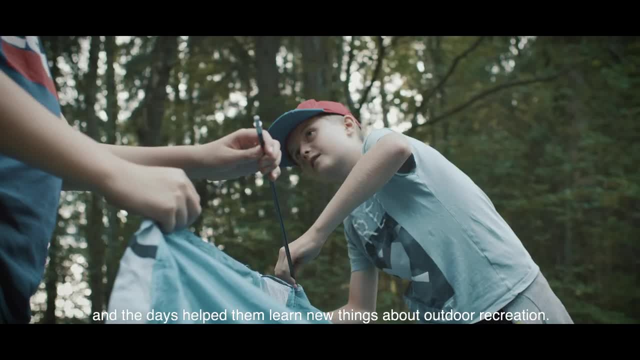 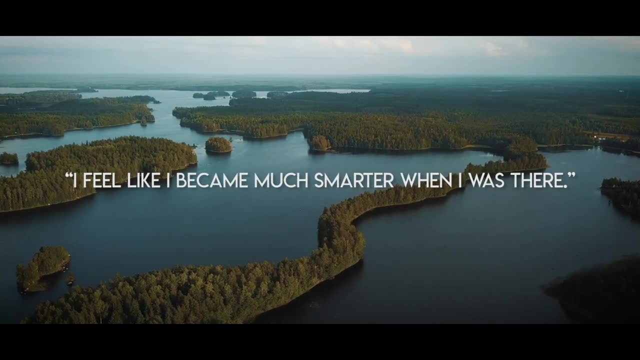 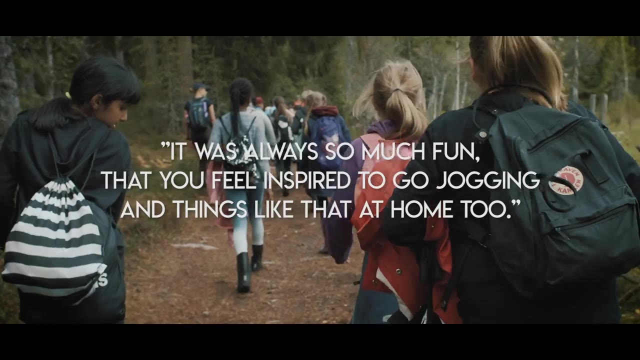 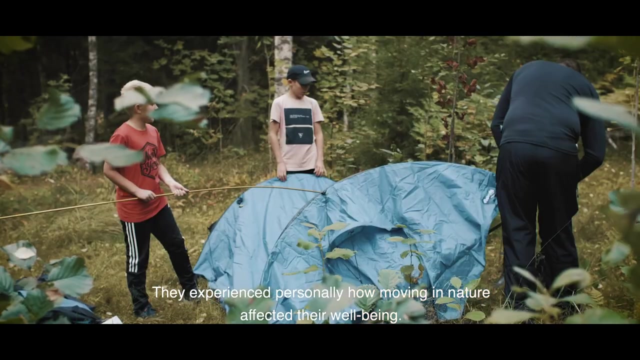 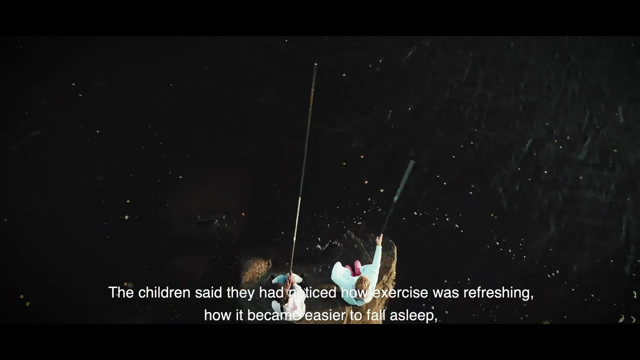 activities and the days helped them learn new things about outdoor recreation. All this inspired them to go out into nature also on other days. they experienced personally how moving in nature affected their well-being. The children said they had noticed how exercise was refreshing, how it became. 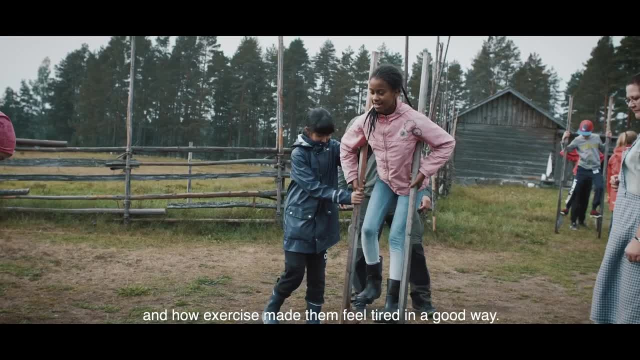 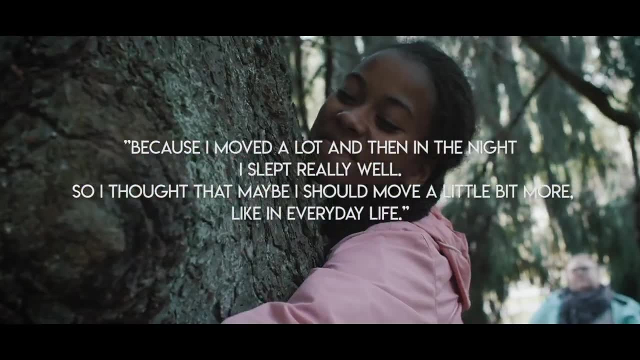 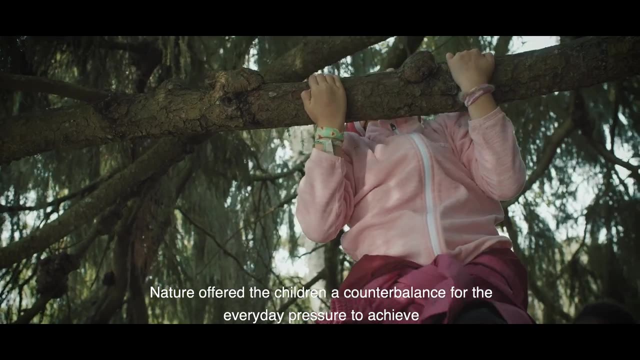 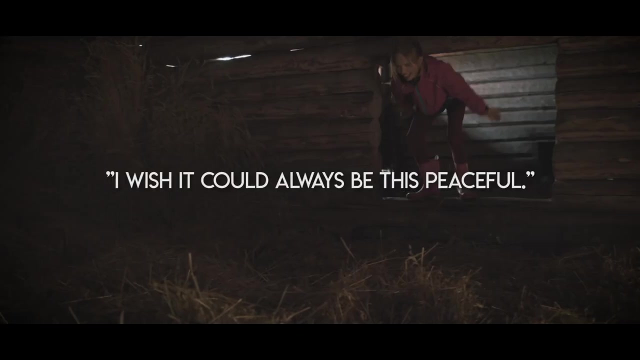 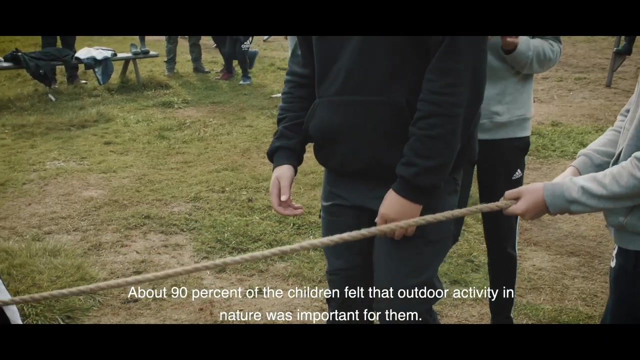 easier to fall asleep and how exercise made them feel tired in a good way. Nature offered the children a counterbalance for the everyday pressure to achieve and to static sitting and to the noise and bustle of daily environments. About 90% of the children felt that outdoor activity in nature was important. 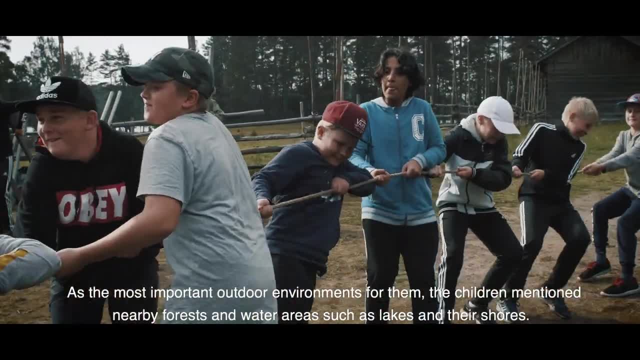 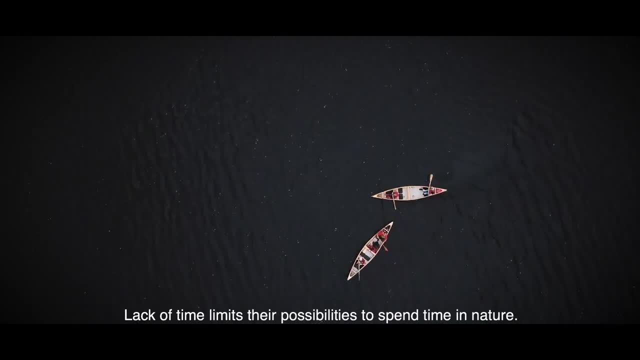 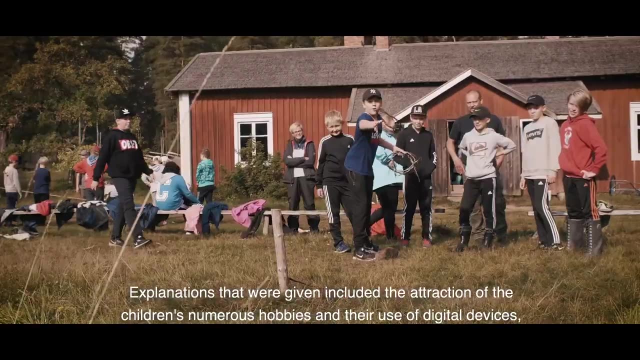 for them. As the most important outdoor environments for them, the children mentioned nearby forests and water areas such as lakes, and their short Lack of time limits their possibilities to spend time in nature. Explanations that were given included the attraction of the children's numerous hobbies and their